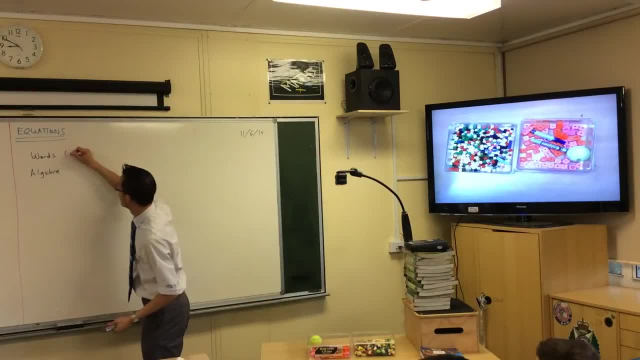 that when you put together a whole bunch of words, we call that a sentence. Is he going to come in? Come in, take a seat. When you put a whole bunch of words together, take a seat there. Take a seat there. 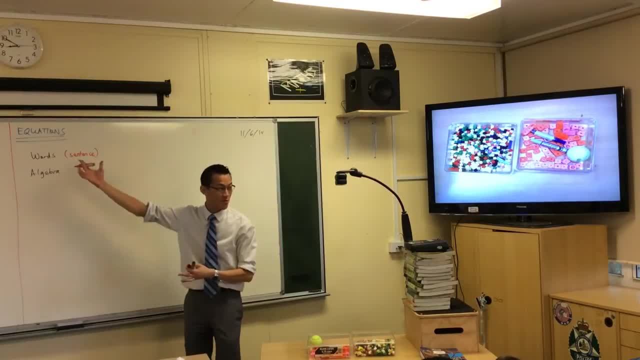 You get a sentence right Now, be very, very careful- We talked about this before- When you put a bunch of algebra and numbers together. right, there was a special word, and it wasn't this one that also started with E Here: Expression, Expression. Well, 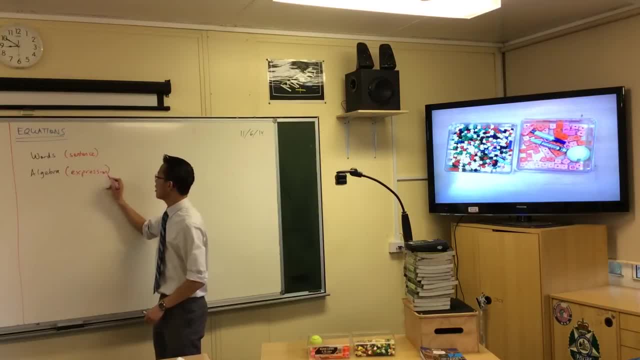 done. Now, this is really important. You remember, I said because a lot of people said: oh, you know, when you put a bunch of algebra numbers together you get an equation. Well, sometimes you do. I'll talk about what that is in a second. but 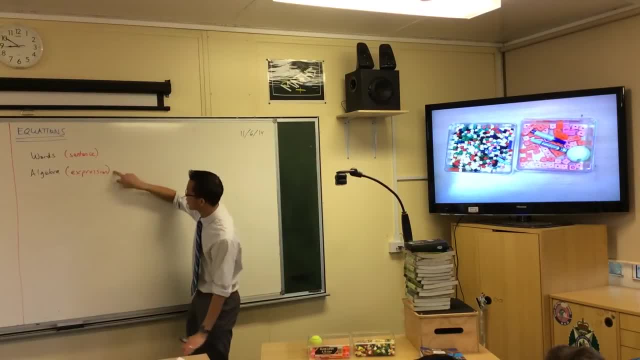 sometimes you don't right. What is the difference between expression and an equation? Yes, Uh-huh, An expression doesn't have an equal sign. Okay, good, So this one doesn't have an equal sign where, as this one does, And the 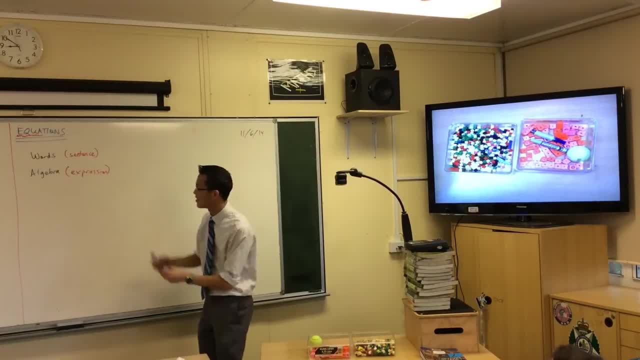 way you can tell is because the word equation- it has it almost- has the word equal in it, Right, Okay, so here's the idea. right, This is what you want to have there. You put words together, you get a sentence. When you put algebra and numbers together, you get an expression. but but, and again sometimes you go: ah, that's because there's not that much value to the word equation, right, You gave it an expression. You know people don't? You don't take that kind of the answering text one-by-one. 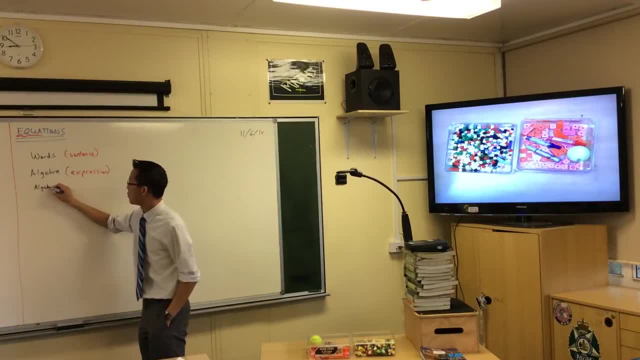 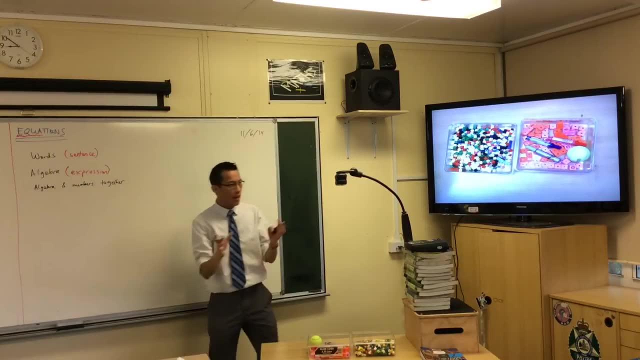 But if the algebra and numbers together, if the sentence that we put together includes something like: all of this stuff, this algebra and numbers is equal to or is the same as or equivalent to all this other algebra and numbers. that's what makes an equation. 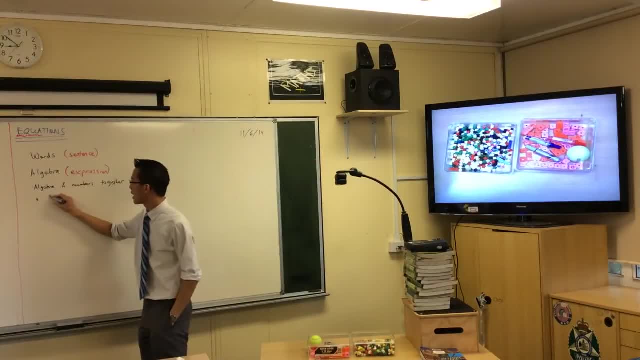 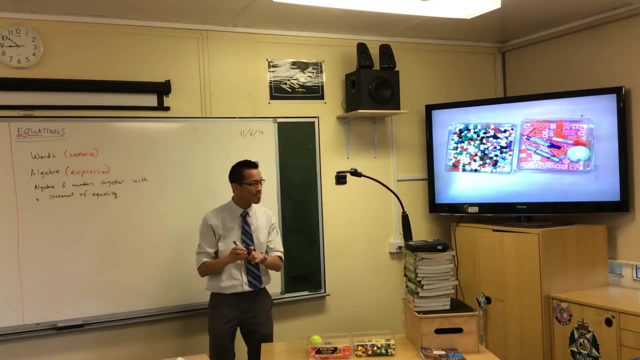 So, together with what I'm going to call, that is a statement of equality, In other words, I'm saying this thing and this thing, they're equal And that's why we use an equal sign. So algebra and numbers, together with a statement of equality, gives an equation.